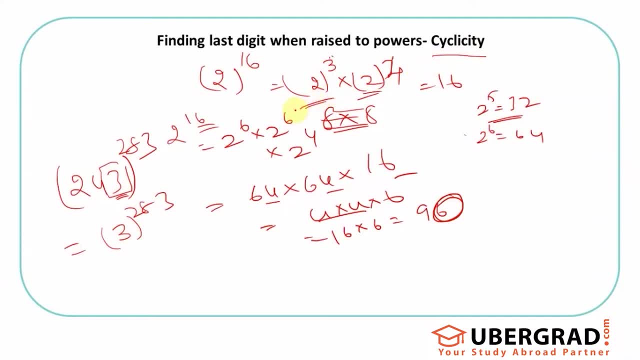 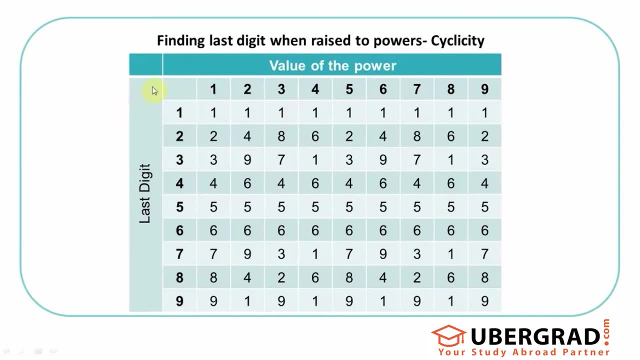 cyclicity. right. there's a behavior you see in this and we use that to solve the problems. Don't be scared looking at this table. I'll explain so that will actually make it easy to understand. So what we see here: 1, 2, 3, these are the units. it just taken 1 to 9, and these are basically raising the powers. like this is fundamentally 1 power 1, is this 1. power 2, is this 1. power 3, is this? 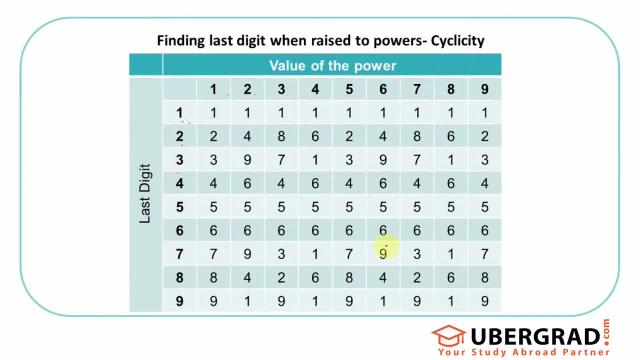 So we have written only the units digit in all the places, right? so let's just go about 2,, right? so this one is 2 power 1 is 2, which is what the units digit you're seeing. this one, 2 power 2, is 4,, which is what we have written. this one is 2 power 3, 2 power 3 is 8,. this one is 2 power 4 is 16, so we have picked the last digit. so we have written 6, 2 power 5 is 32, so the last digit is 2, we have written 2.. 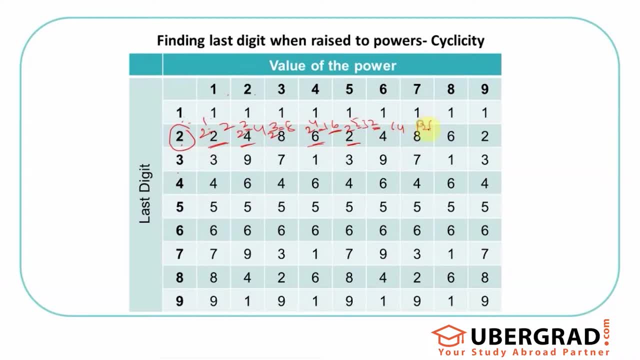 Right, then 2 power 4 is 64,, 128,, 256,, 512,. so the last digit is 2, 6,. see, that's what we have written right. the same case for every. so this is basically 4 power 1,, 4 power 2,, 4 power 3, and the last digits. 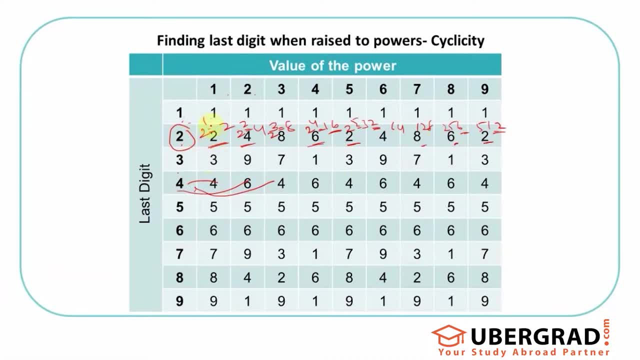 So let's focus on the 2 again. see the first 2: power 1, the units digit is 2, then I'm getting 4, then 8, then 6, and then again I'm seeing 2, right, and then again I'm seeing 4.. 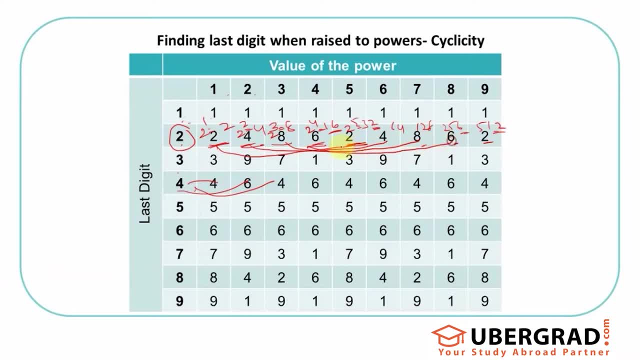 Then again I'm seeing 8, again I'm seeing 6,, and again I'm seeing 2, so 2 power 10 would be 4, 2 power 11, 8, 6, and so on. right, it keeps going on, it repeats for every digit. let's look at 7 for a sec. 7 power 1, 7, 9,, 3,, 1,, again 7,, again 9,, again 3,, again 1,, right. 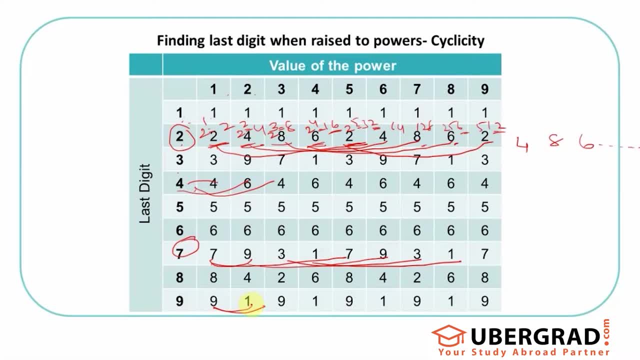 You see, for 9, 1, 9, 1,, 9, 1,. yes, repeating only every two times. right here i am seeing the repetition happening every four times: seven, nine, three, one. seven, nine, three, one, seven, nine, three, one. but everything you see is max. 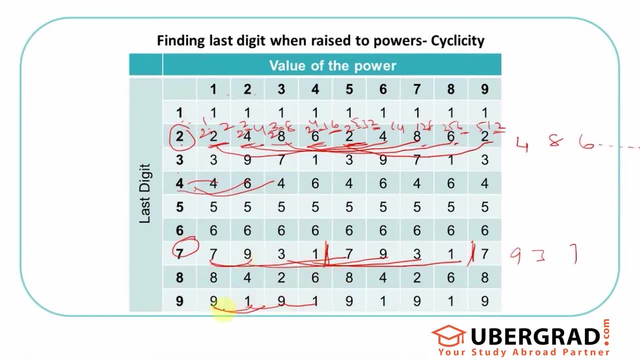 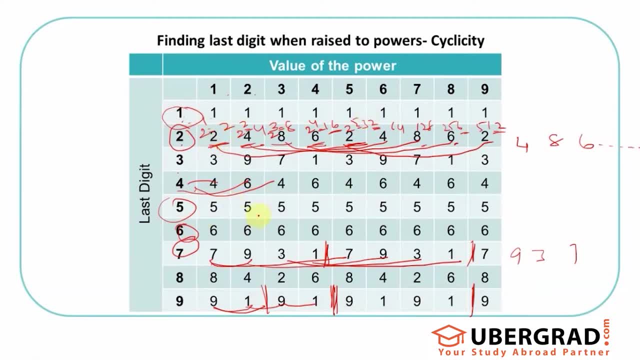 one, one, one, five, five, five, power one, five, power, two. all times you get the same units to set, right. so this is basically called the cyclicity concept. that's fundamentally the repetition, the pattern we are seeing, right, it's repeating every four times, right, so there's a four bars. i am seeing the repetition starting. so how do we use that? let's get to that. 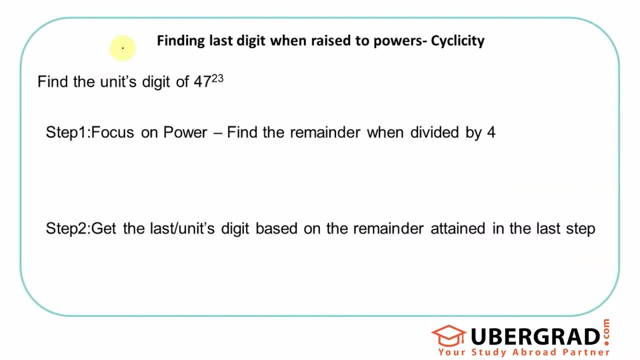 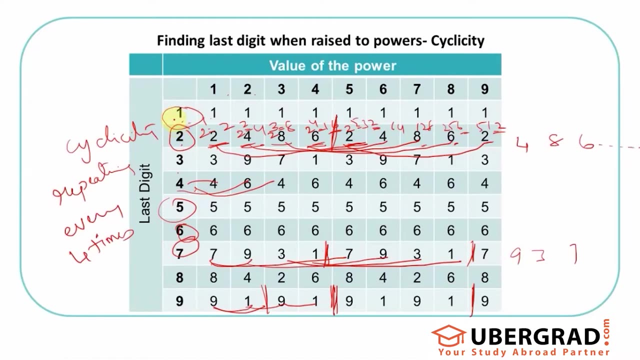 with an example right, if you ever see a question asking you: right, 47 power 23. this is fundamentally asking you to find 7 power 23 right. so first, what we need to do is because you have seen the repetition happening: every like powers, like every fourth power right. like two power one. 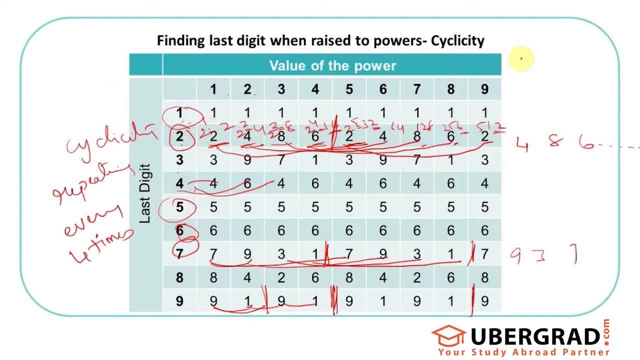 so that's let me write this here, right, right. So 2 power 1 is same as 2 power 5 is same as 2 power 9.. Similarly, 2 power 2 is same as 2 power 6 is same as 2 power 10, right With respect to the last digit, 2 power. 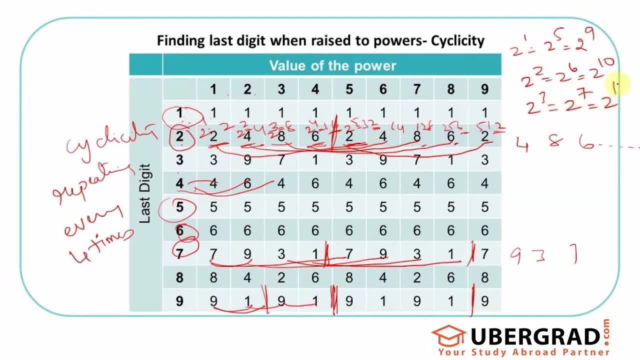 3 is same as 2 power, 7 is same as 2 power 11, and so on. right, 2 power 4,, 2 power 8 and 2 power 12.. You see 1 plus 4, 5,, 5 plus 4,, 9,, 2 plus 6, 4,, sorry, 6 and 6 plus 4,. 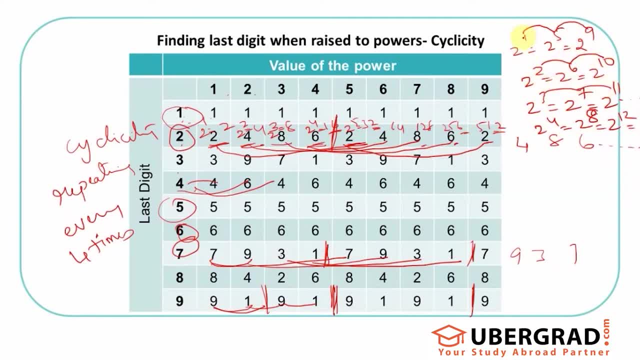 10.. 3 plus 4, 7,, 7 plus 4, 11.. And you see, this is fundamentally adding 4 to the powers to get the same last digit right: 2 power 1 is 2, 2 power 5 is 32, again 2, 2 power. 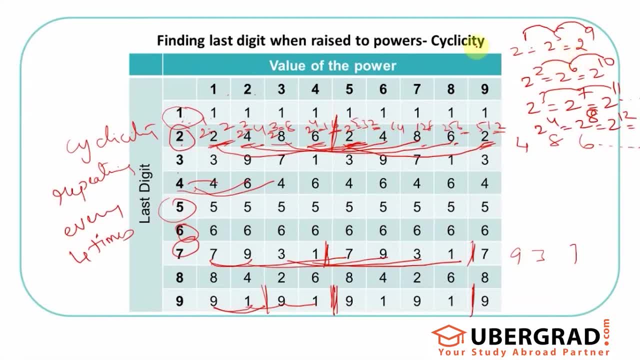 9 is 512, again 2.. That's what we are seeing, So all I need to focus is on the powers right Divide with the 4, whatever. the reminder I am getting would give me a clue about what should be the last digit right. 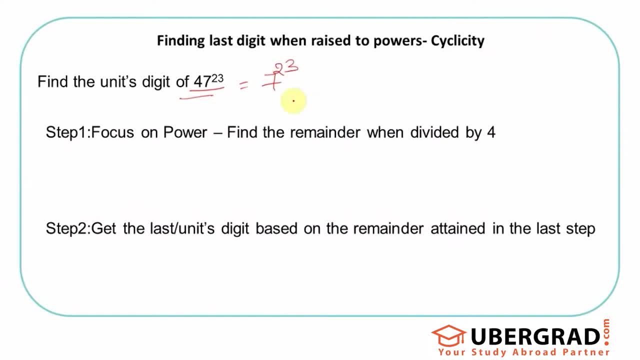 Let's say again, using the same logic: right. The steps to do follow is focus on the power first right. So the power is 3, right 23 divided by 4, what would be the reminder, Equal to 1 multiple of 4 is: 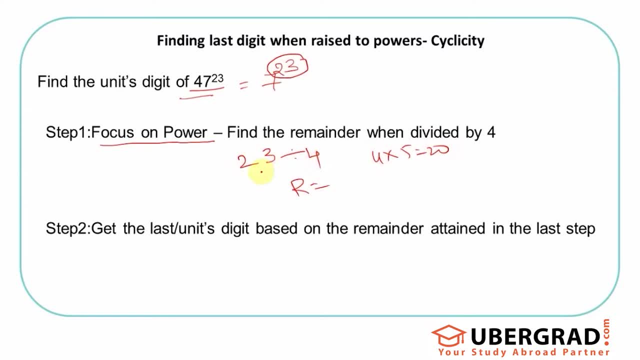 4, 5 is 20, right. 4, 6 is 24, is greater than 23,. right, So the reminder is 3, right, Once you know, the reminder is 3,. so that means 7 power 23 is same as 7 power 3 in terms of. 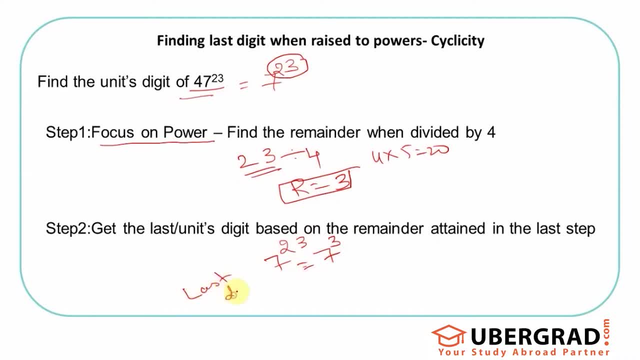 the last digit Right 7 cube is 343, so I know the last digit is 3.. So the last digit of 47 power 23 is also 3,. right, Let's say if the question was 47 power 29,. okay, Just for our understanding. 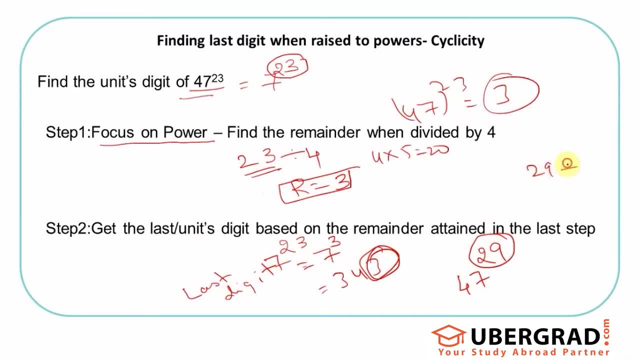 So again, focus on the power 29 divided by 4, the reminder is 4, 7, 7, 28 is the closest multiple, so the reminder is 1.. This is same as 7 power 1 in terms of last digit, so it's 7, so the answer is 7. for this right That. 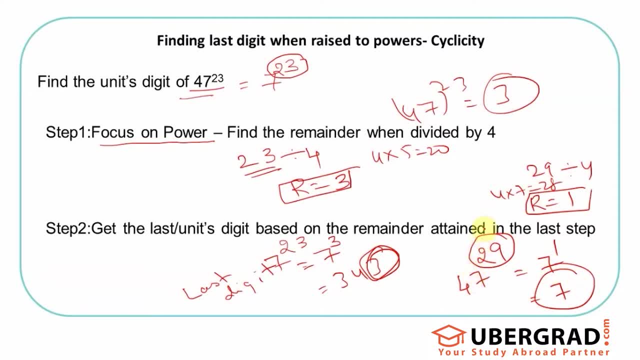 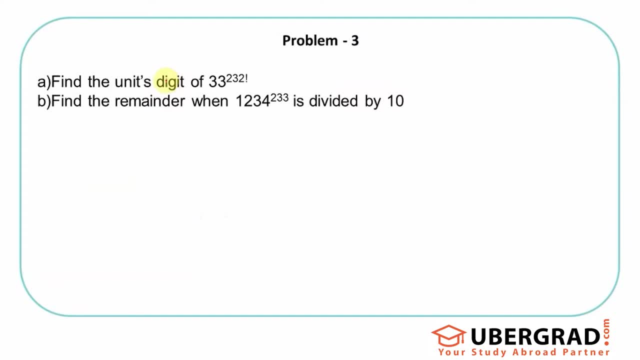 is how you will solve the questions for the last digit, or unit's digit, focusing on with respect to the powers, right? So this one is something related to the powers. It's asking you to find the unit's digit of 33 raised to 232 factorial, So 232 factorial means. 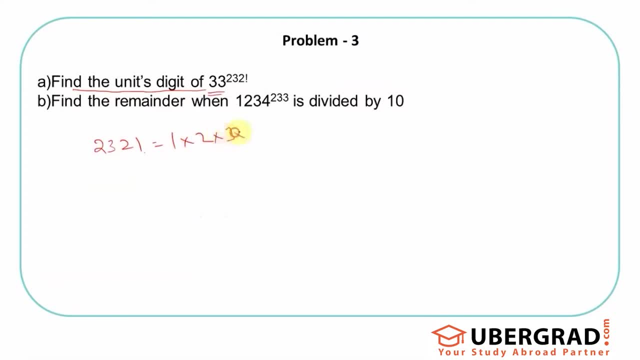 basically 1 into 2, into 3, into 4, into, so on, up to 232, right. So, as I said, the first step is find the reminder when the power right, 232 factorial is divided by 4, because 232 factorial is basically 1 into 2, into 3, into 4, into everything. So 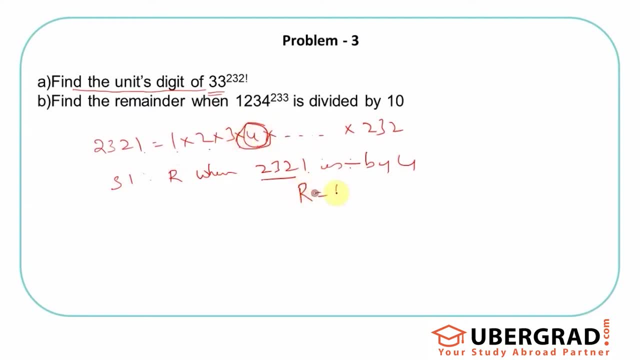 when I divide by 4, the reminder will be automatically 0, right, So that means 33 power 232 factorial a is same as 3 power 232 factorial is same as 3 power 4 and not 3 power 0. okay, because the